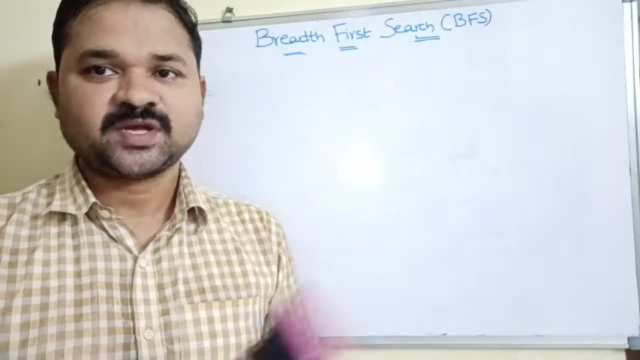 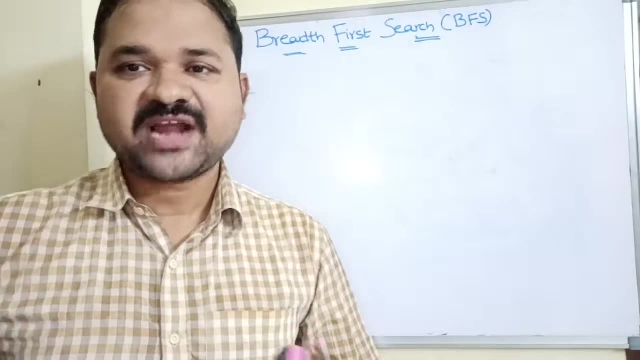 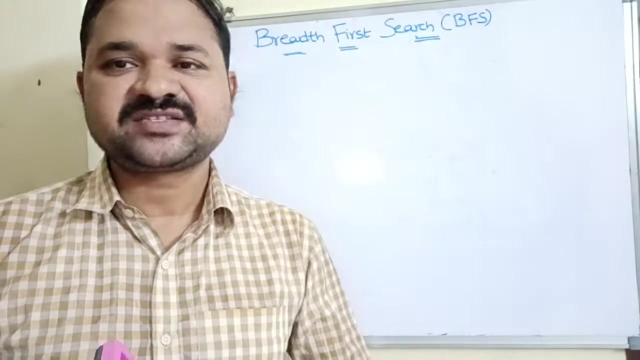 Now let's see about breadth of assay. In short, we can call it as BFS. BFS is a graph traversal technique. Graph traversing means visiting the nodes or vertices of the graph. We can mainly traverse the graph in two ways. The first way is breadth of assay and the second way is depth of. 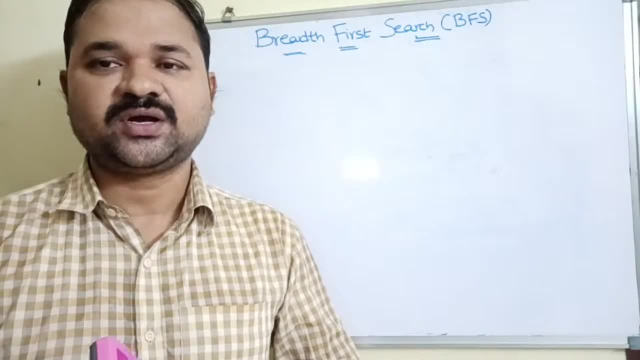 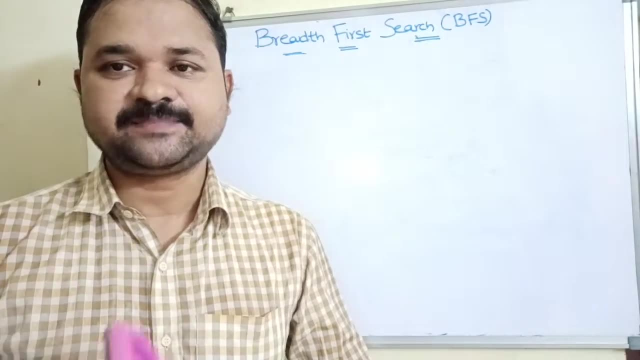 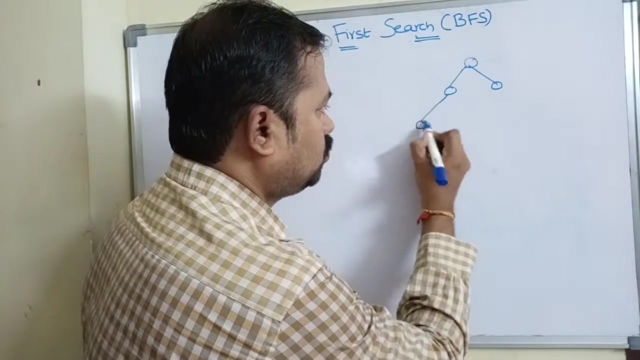 assay. In this video we are going to discuss about how we are traversing a graph with the help of the breadth of assay. BFS means level by level searching. Let us assume that we have a graph like this. So let the vertices or nodes are arranged like this. So this is nothing but. 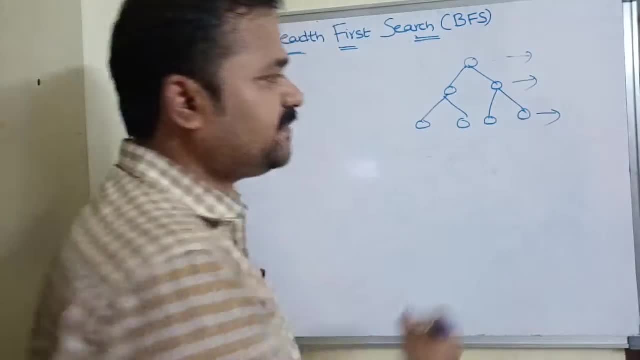 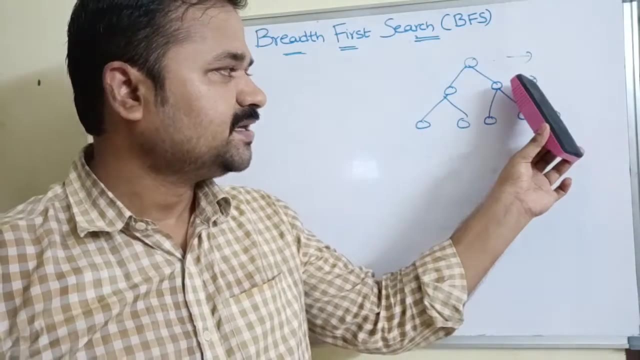 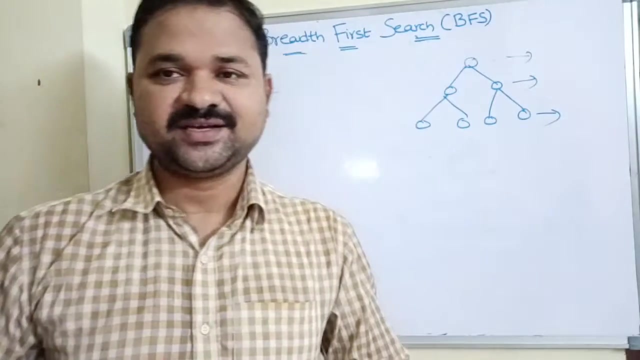 level 0, this is nothing but level 1, this is nothing but level 2.. So first the nodes that are at level 0 are visited first, and then the nodes that are at level 1 are visited, And then the nodes that are at level 2 are visited. So, likewise, breadth of assay will be. 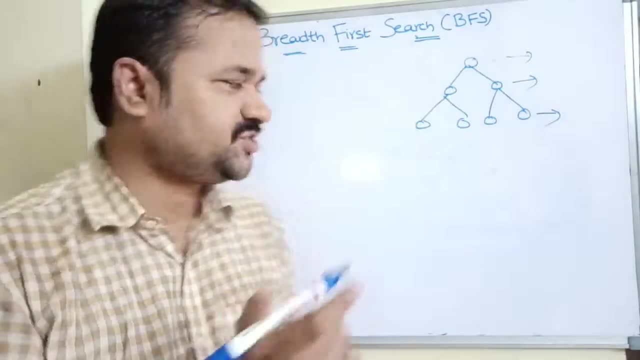 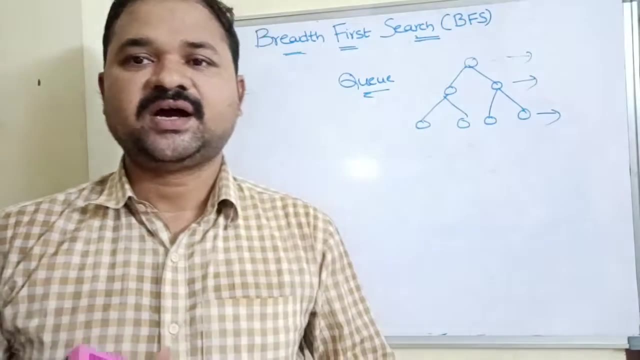 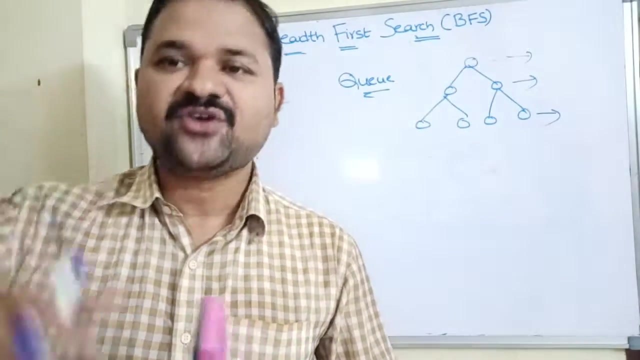 done In order to implement the breadth of assay. we use a data structure called Q, So we know how Q will work. Q will work on the principle of FIFO: first in, first out. Insertion should be done from the end of the Q. that is nothing but variant Variance. deletion should be done from beginning. 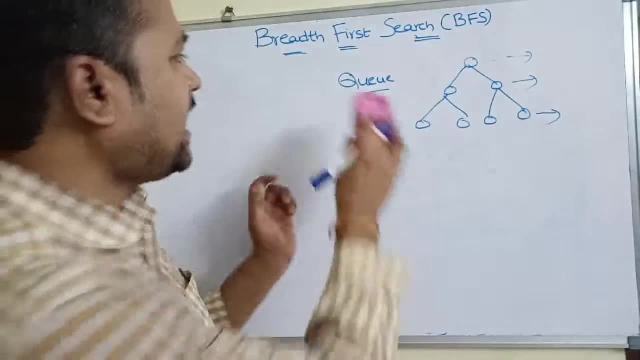 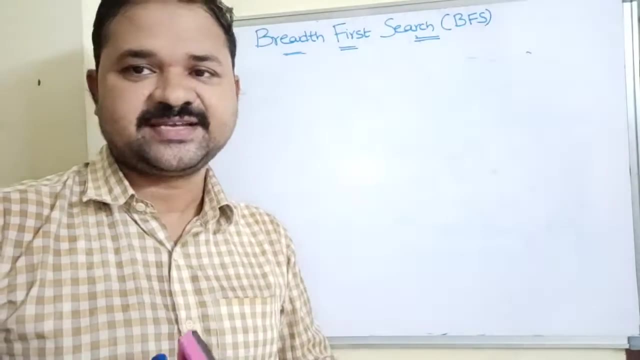 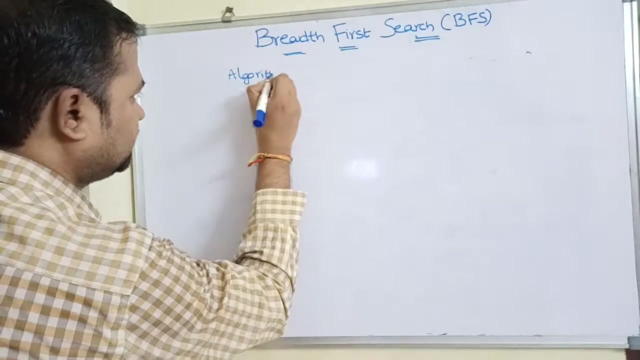 to end of the Q. that is nothing but front end. First let us see the algorithm for the breadth of assay And then, with the help of an example, we will demonstrate breadth of assay in detail. So let us see the algorithm. So let us see the algorithm for the breadth of assay. So let us 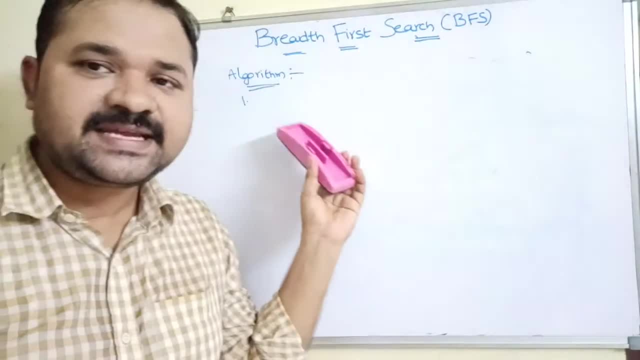 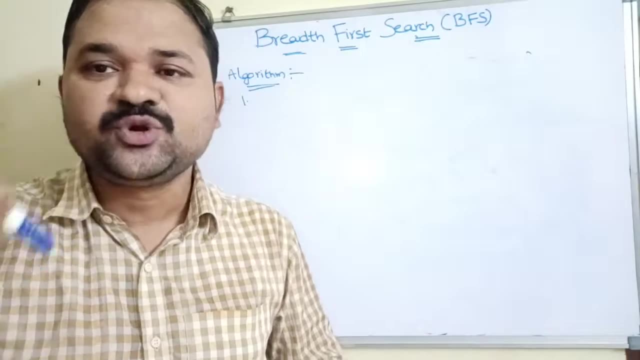 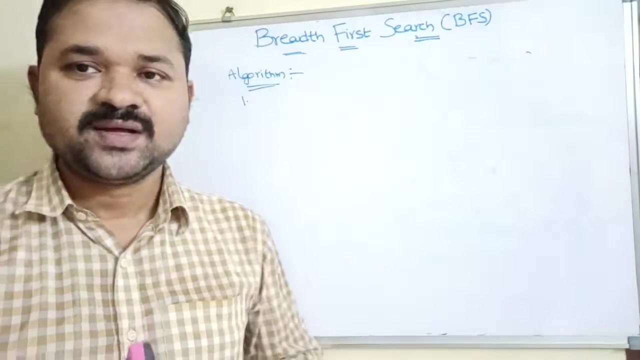 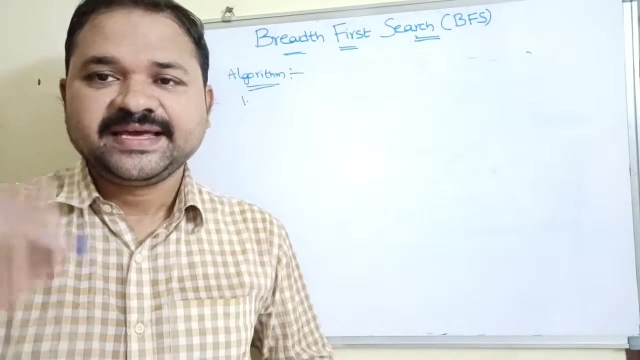 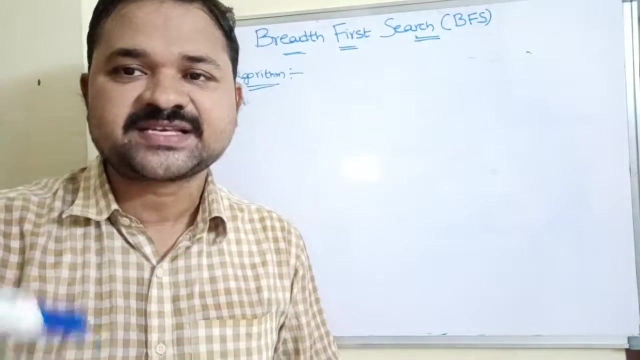 see the first step: Select any vertex as the starting vertex, Insert that vertex into the Q and make the status as visited. So what is the first step here? We have to select any vertex as the starting vertex and insert that vertex into the Q and make the status of that vertex as visited. 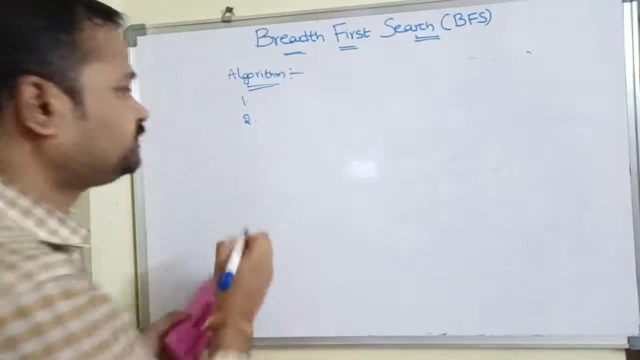 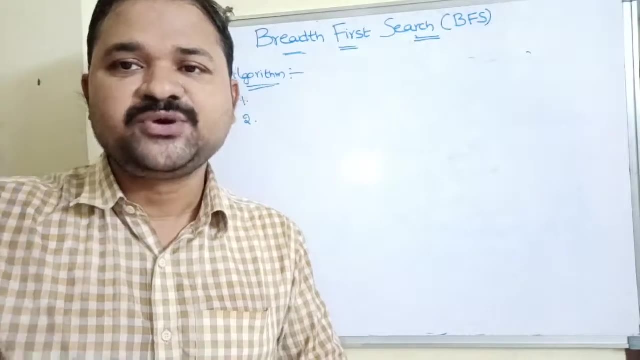 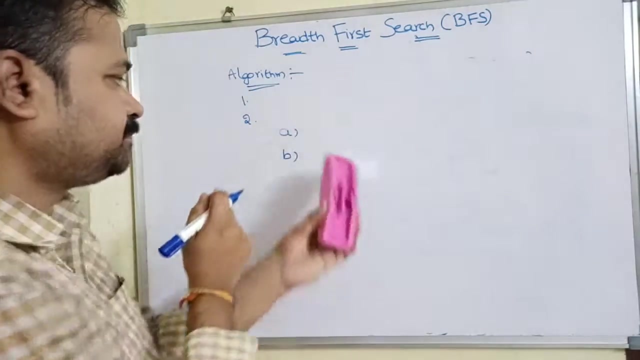 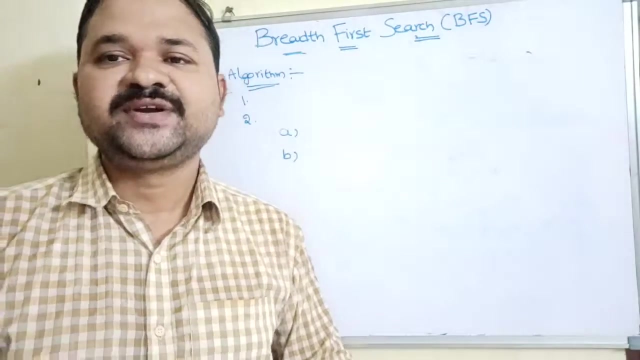 So that is the first step. The second step: while the Q is not empty, while the Q is not empty, then we have to perform two steps, A & B. so let us see the first one: Delete a vertex from the Q and display it. So display it is nothing, but we are traversing that vertex, we are visiting. 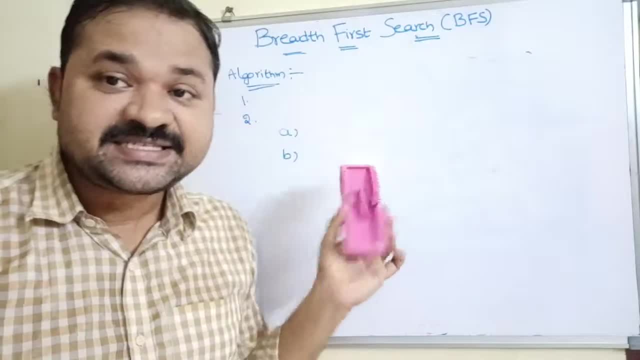 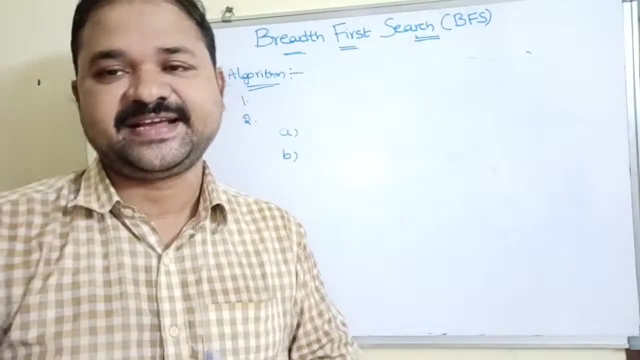 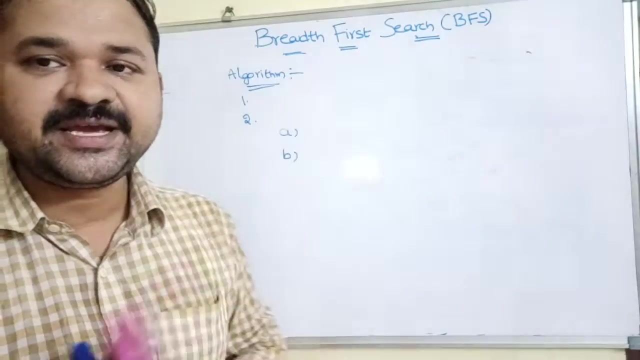 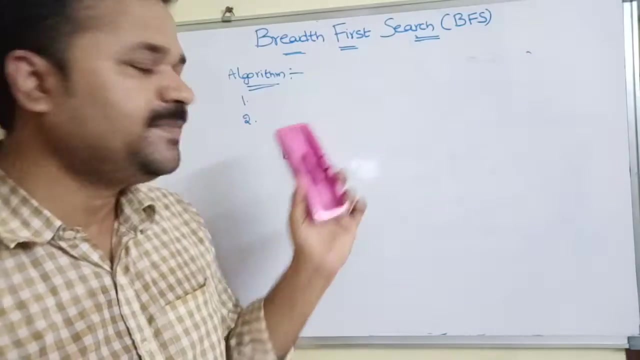 that vertex And the second step is insert all the un-visited adjacent vertices of that vertex- deleted vertex- into the queue and make the status as visited. so what is the second step here? while the stack is not empty, then we have to perform two things. so what is a bit? delete a. 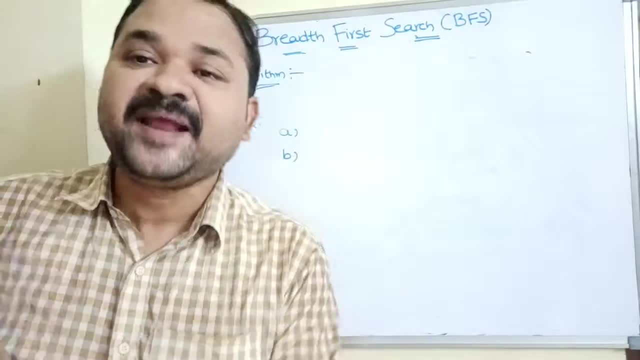 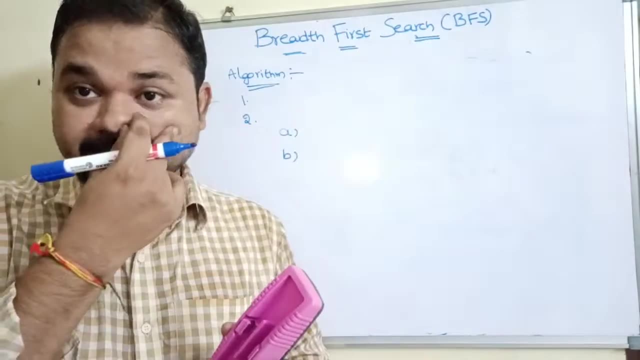 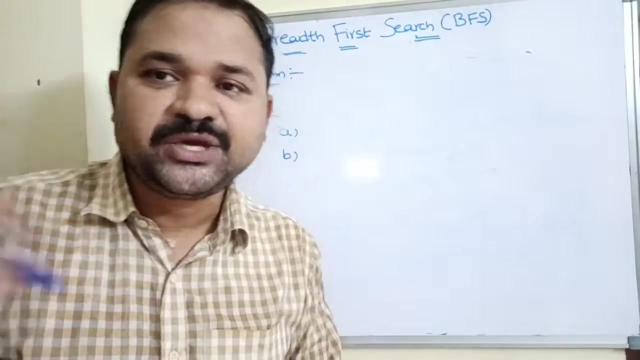 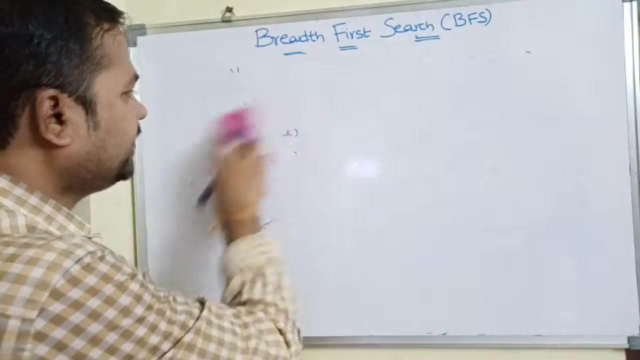 vertex from the queue and display it. we know that delete- deleting- should be done from the front end, and b step is insert all the unvisited adjacent vertices of that vertex into the queue and make their status as visited. okay, now, with the help of an example, we try to demonstrate bfs algorithm. 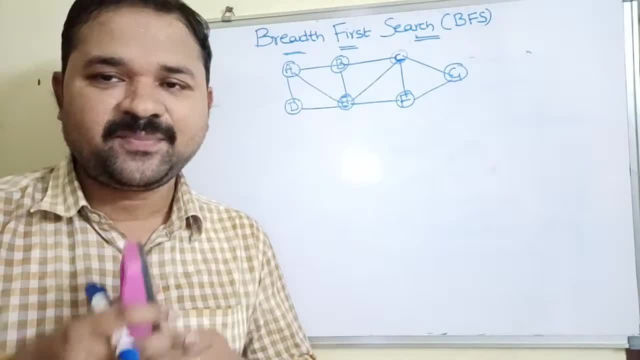 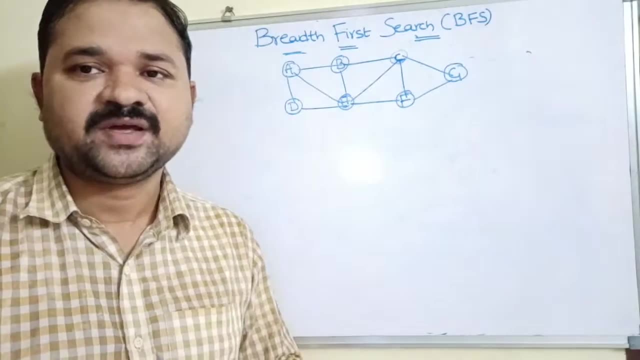 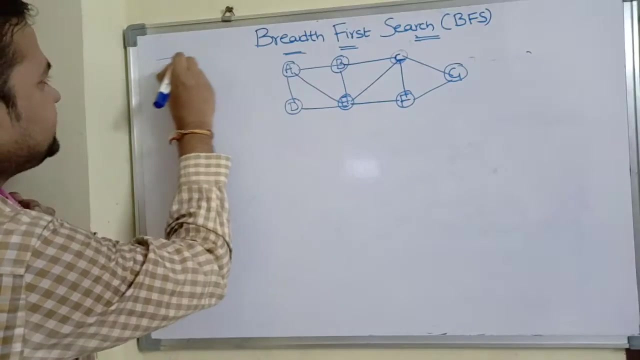 let's see the first step. what is the first step? we have to select one of this vertex as a starting vertex, insert that vertex into the cube and make the status as visited. so totally, here we have one, two, three, four, five, six, seven nodes, and let us assume that this is our visited vertex matrix, our array. 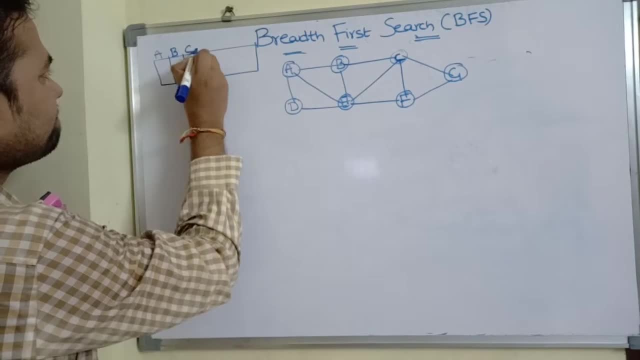 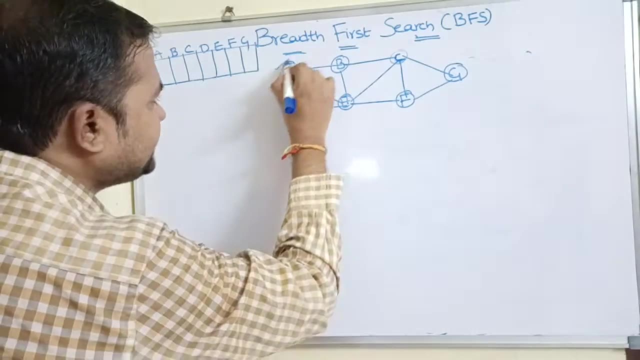 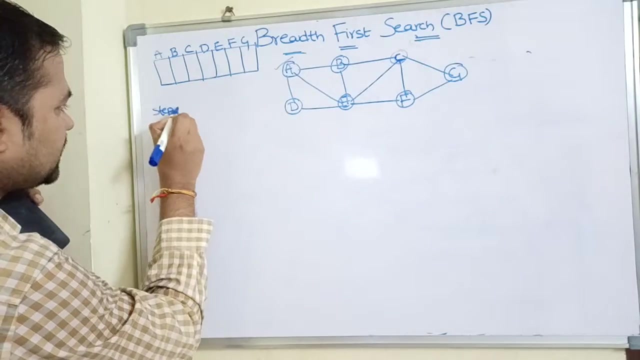 so here we have seven nodes: a, b, c, b, e, f, g, seven nodes. let us assume that a is the starting vertex, so we have to insert that vertex into the cube. so let us take step one, step one. uh, here we have a stack. i'm sorry, which data structure we are using? q? 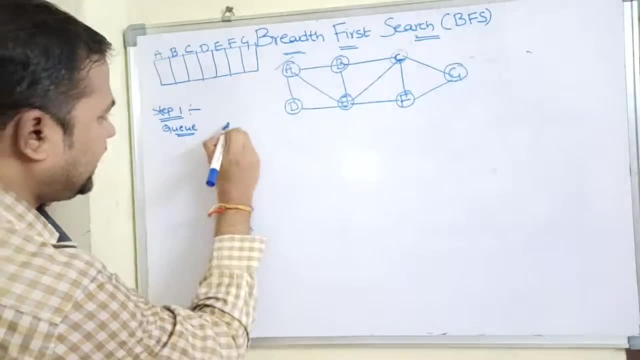 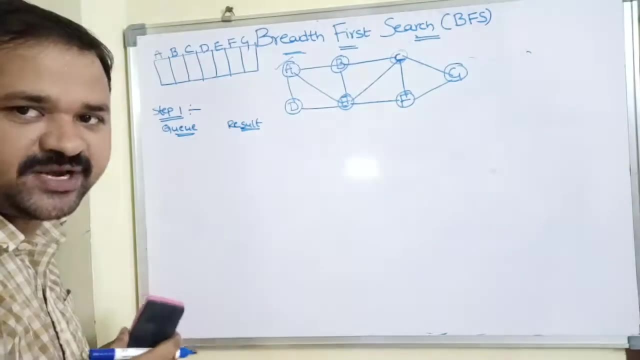 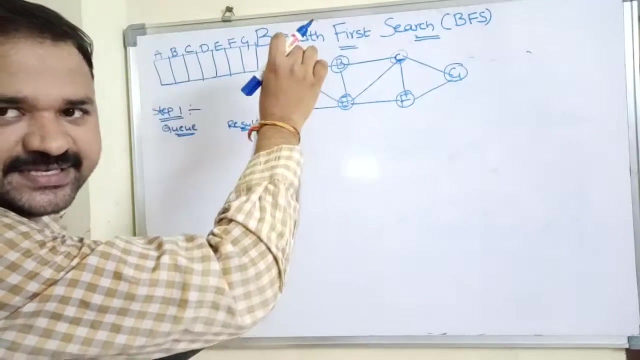 data spectra. so this is nothing but q and result. so that means which vertex we visited. okay, so initially let us assume that a is the starting vertex, so insert: a is the starting vertex. so after that, what we have to do, we have to insert that vertex into the queue and make the status as 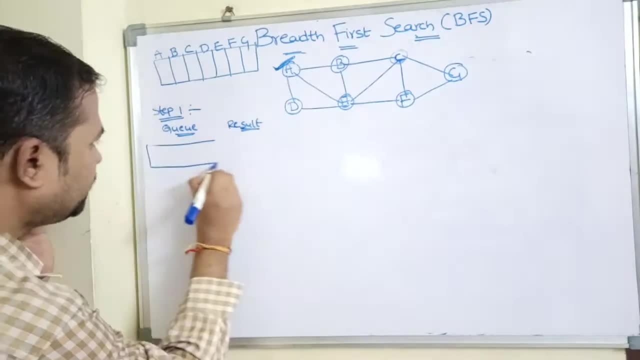 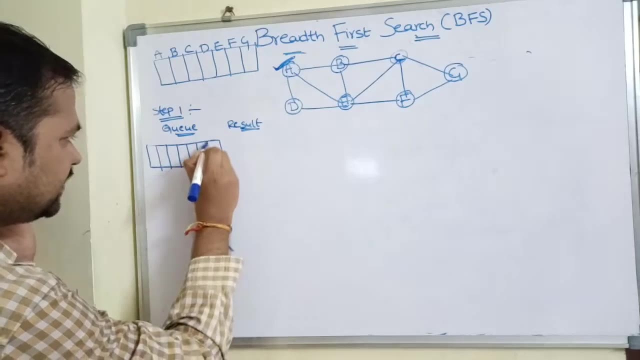 visited. So totally, how many nodes are there? So totally, our cube can store 7 nodes. So 1,, 2,, 3,, 4,, 5,, 6,, 7 nodes. So here, what is the starting vertex? we are assuming, 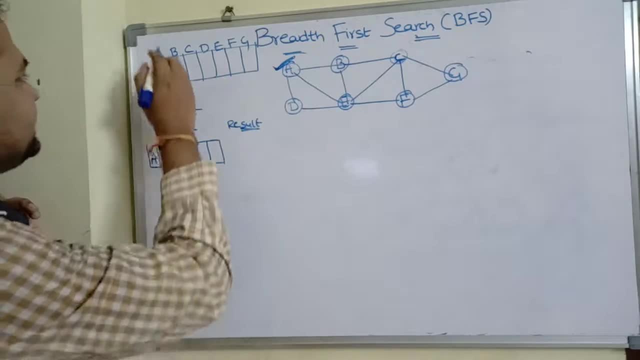 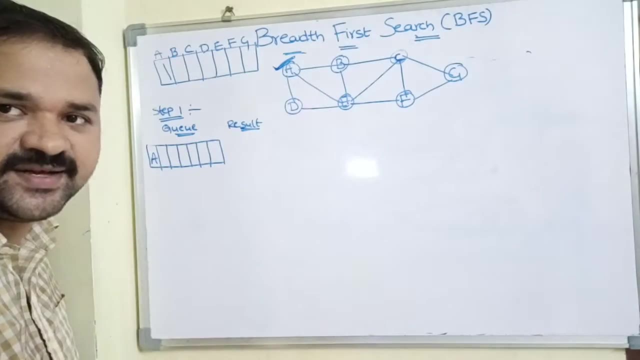 A. So insert A into the cube and make the status as visited. So here the vertex A is visited. So let us assume that 1 stands for visited where A 0 stands for not visited. So till now we have visited only the first vertex. 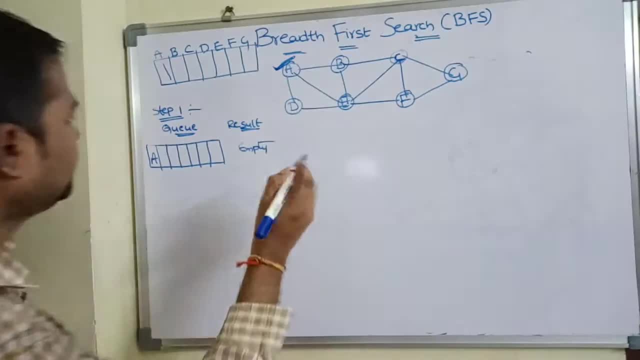 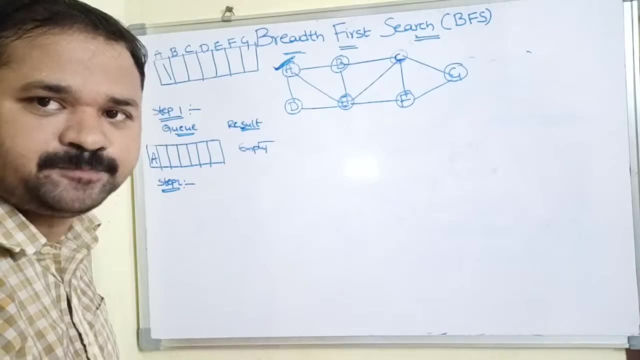 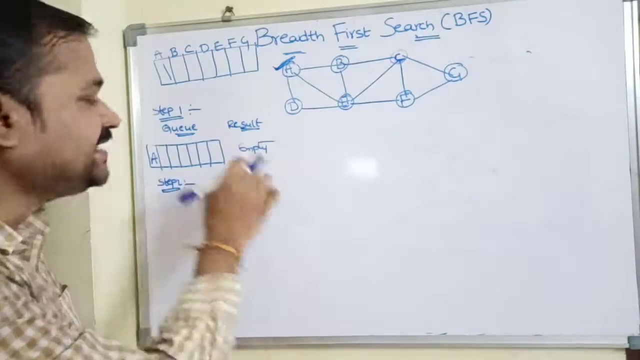 So initially, the result is empty. Now let us take step 2.. So what is step 2? If the cube is not empty? if the cube is not empty, then delete a vertex from the cube and display it. So here, this is nothing but our cube. 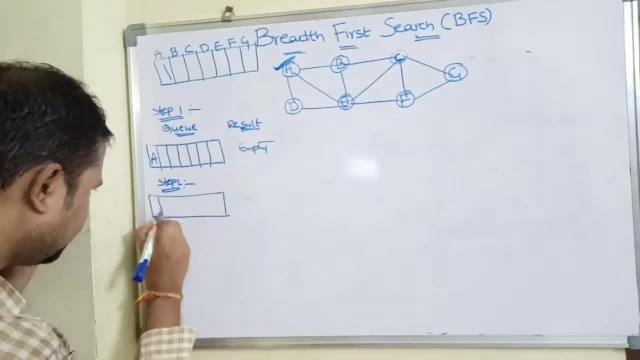 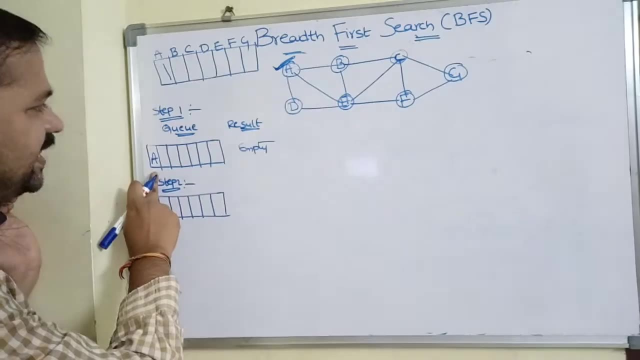 So our cube totally contains how many nodes? 7 nodes. So 1,, 2.. 3,, 4,, 5,, 6,, 7 nodes. So we have to delete A from the cube and display it. 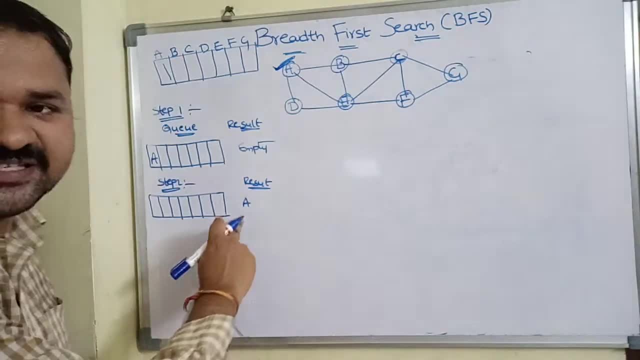 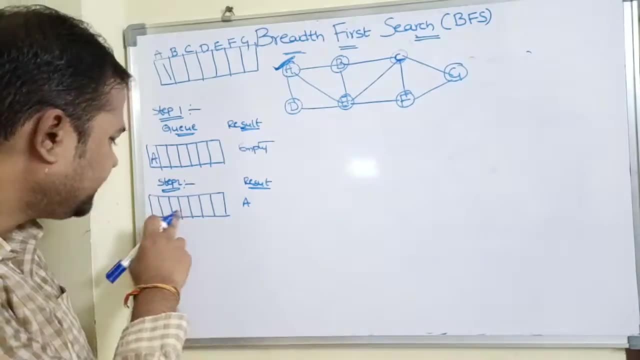 So we are displaying A. So it specifies that we have visited the vertex A. And then what is the b-bit here? In second step, we have two bits While the stack is not empty. then delete an element from the cube and display it. 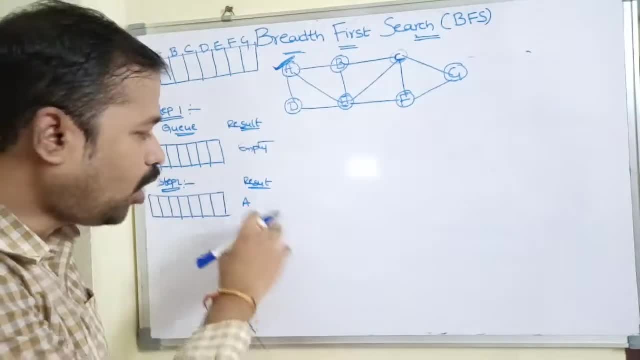 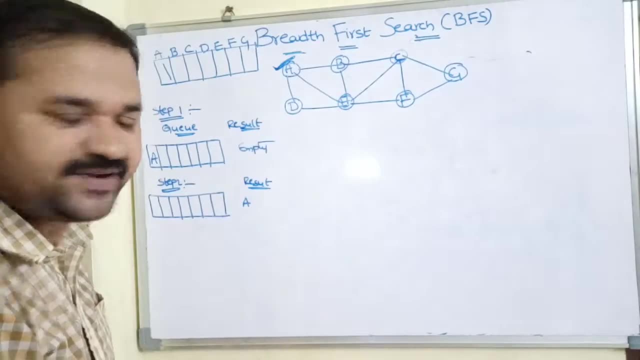 And then we have to insert all the unvisited adjacent vertices of this vertex. And then we have to insert all the unvisited adjacent vertices of this vertex into the cube and make these statuses as visited. So what are the adjacent vertices of A? 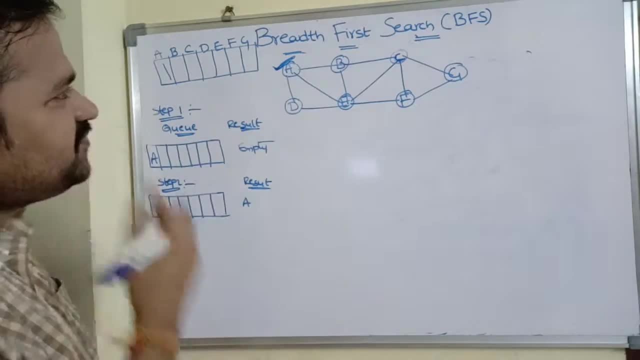 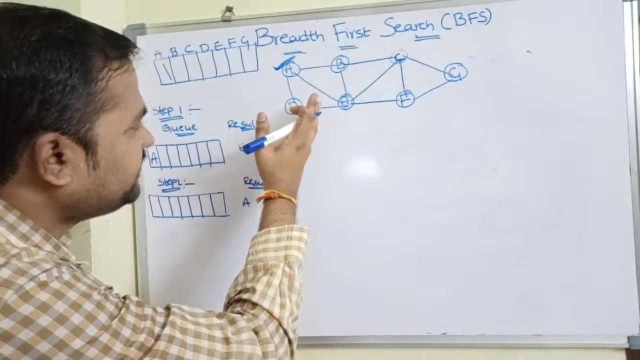 Here we have B as well as D. Here breadth of a set means level by level searching, So level by level searching. So let us assume that this is the first level we are visiting. This is the second level we are visiting. 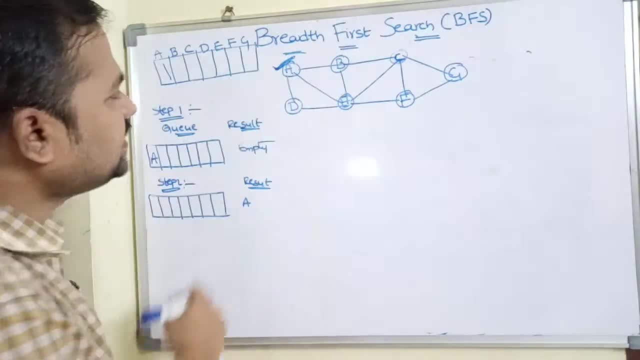 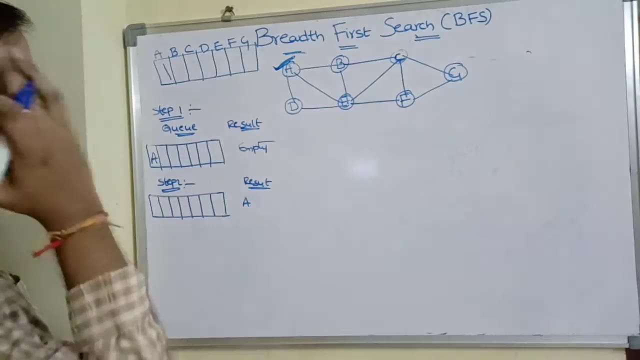 This is the third level we are visiting. So here, what are the adjacent vertices of A, B D E? So B D E are the adjacent vertices. So let us assume that this is level 0.. So first write the vertex D. 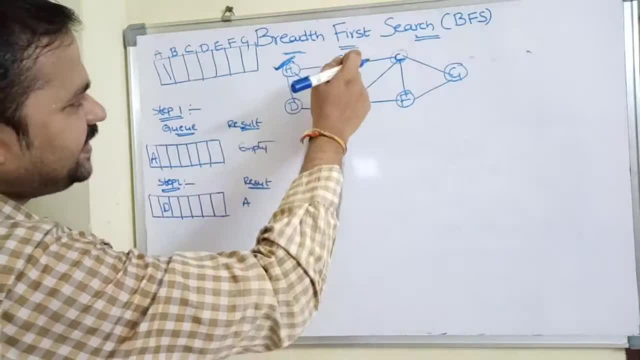 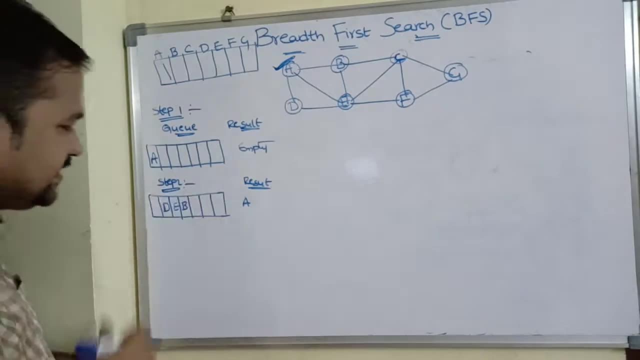 We can write in any manner as we like: So D, Next B, E, or E B, So E B. So the second step is over, So next perform one more step, Step 3.. So what is step 3 here? 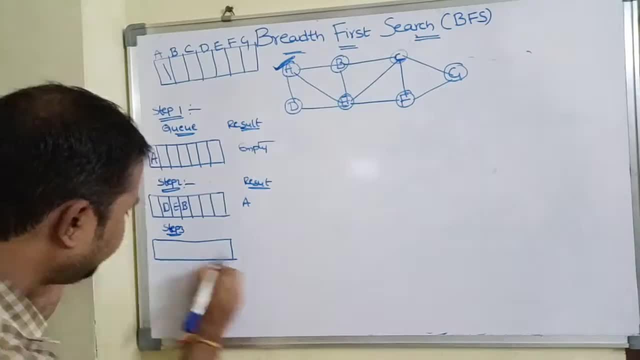 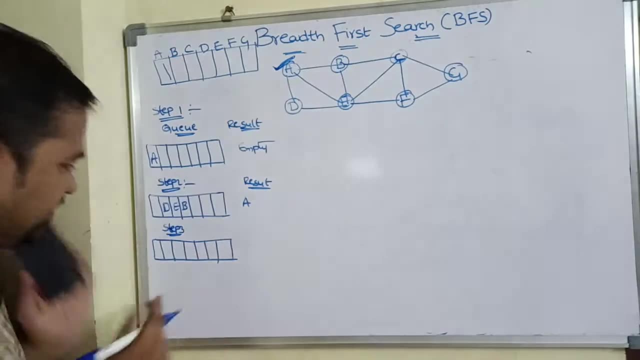 Same, Same process While the cube is not empty. So totally, we have 7 nodes: 1,, 2,, 3.. 4,, 5,, 6, 7.. 1,, 2,, 3,, 4,, 5,, 6,, 7.. 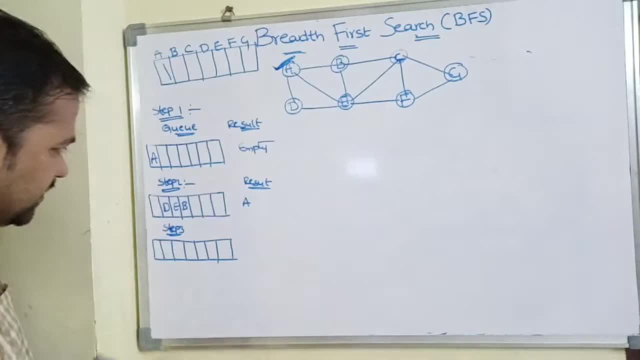 While the cube is not empty. So here the cube is not empty, So delete an element from the cube. We know that deletion should be done from the front end, So this is the front end and this is the rear end. 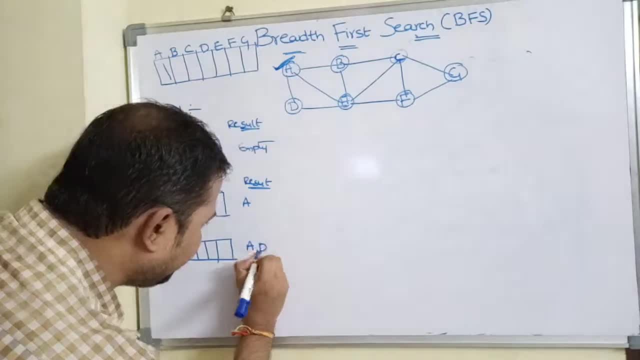 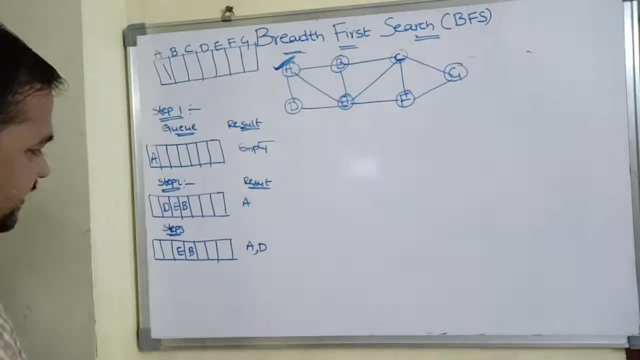 So D will be deleted from the cube And it will be displayed. So next, here we have E and B, Because D is deleted And we have to insert all the here D, E, B are visited. Okay, Okay. 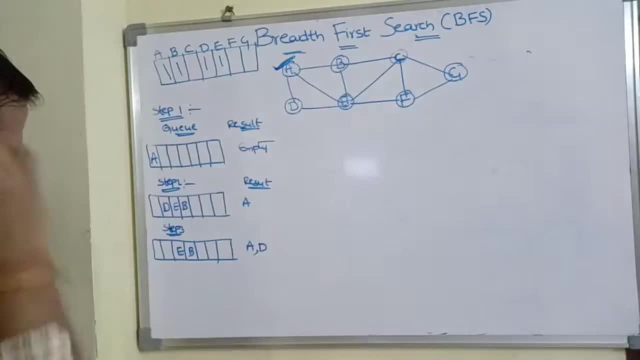 So next we have to insert all the unvisited adjacent vertices of D into the cube. So what are the adjacent vertices of D? We have two vertices. First one is A, Second one is E, But A is already visited as well as E is already visited. 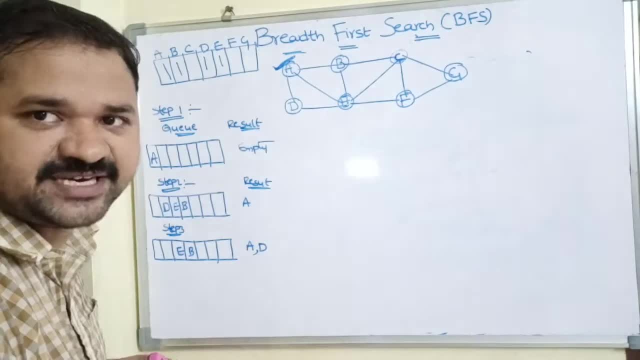 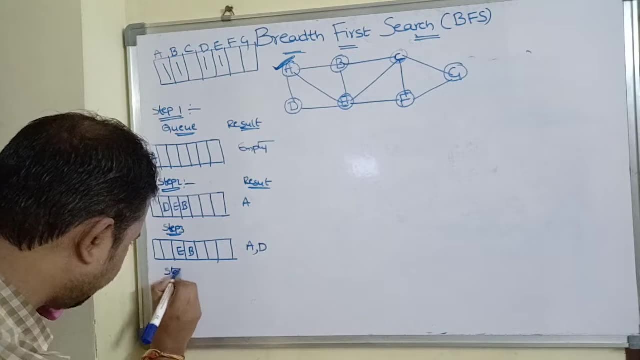 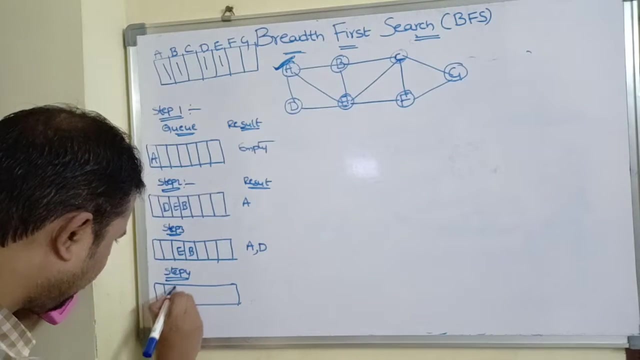 So there is no need to perform any enqueue operation now. Now let us do the next step, Step 4.. Step 4., Step 4.. So what we have to do? First let us write the queue. So totally we have seven nodes. 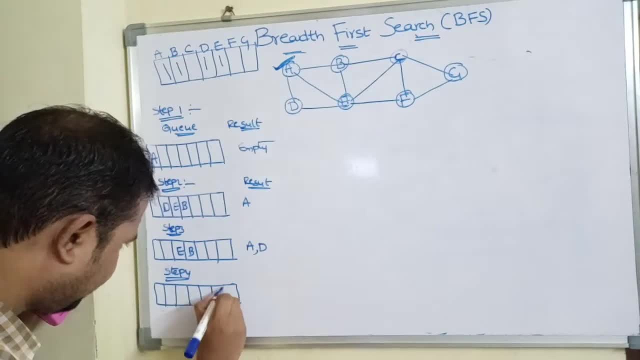 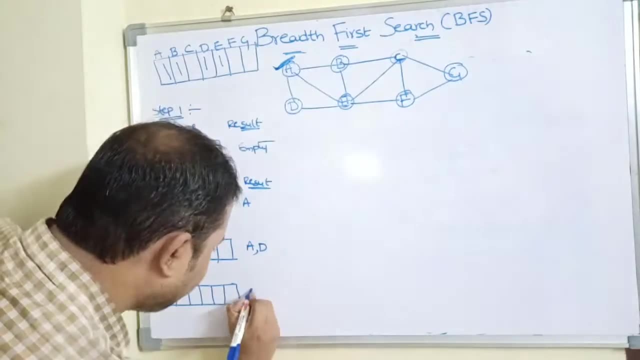 1,, 2,, 3,, 4,, 5,, 6, 7.. Okay, So first we have to delete an element from the cube. So difference is at E location. So delete E from the cube. 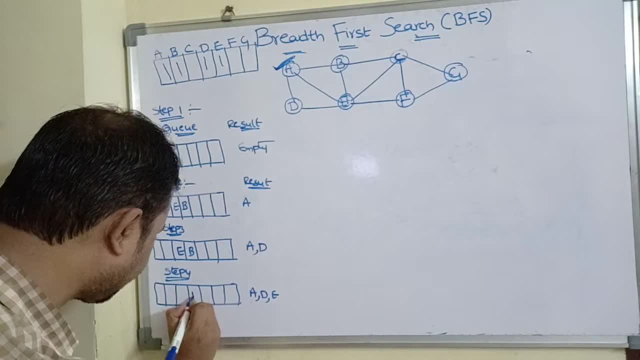 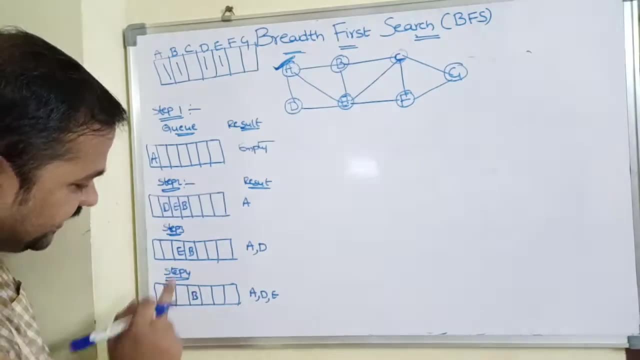 So E is deleted. So what is the next node here? B is the next node. So next we have to insert all the unvisited adjacent vertices of E into the cube. So what are the adjacent vertices of the cube? 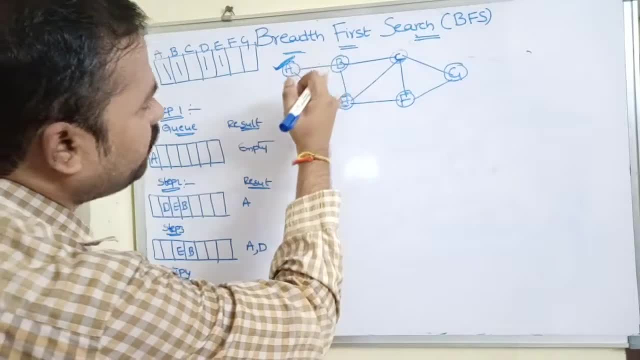 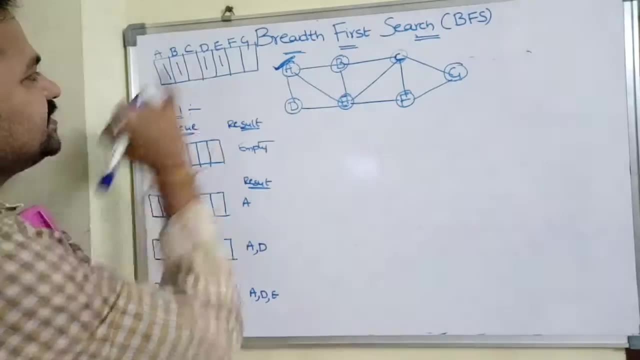 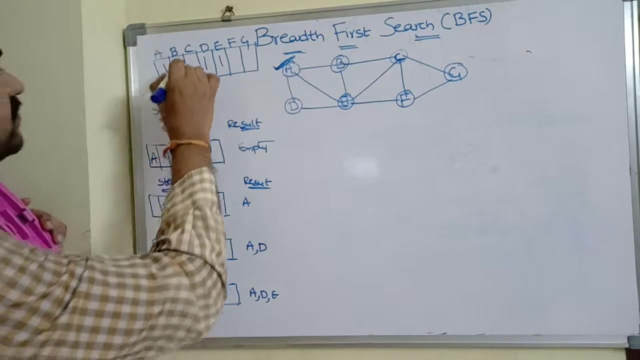 So what are the adjacent vertices of the cube? are the adjacent vertices of the e? we have b, c as well as f. okay, b, c, f. so b is already visited. so c and f are not visited. so let us insert those two nodes into the q, so c and f are visited now. 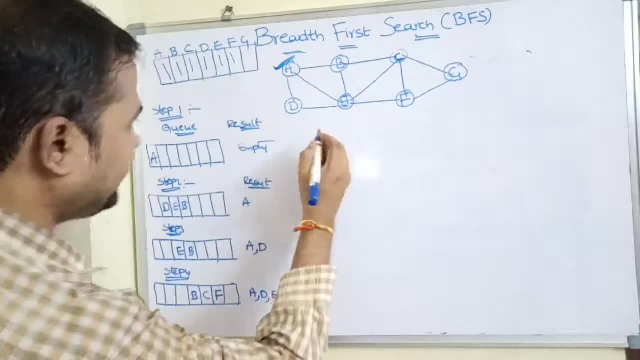 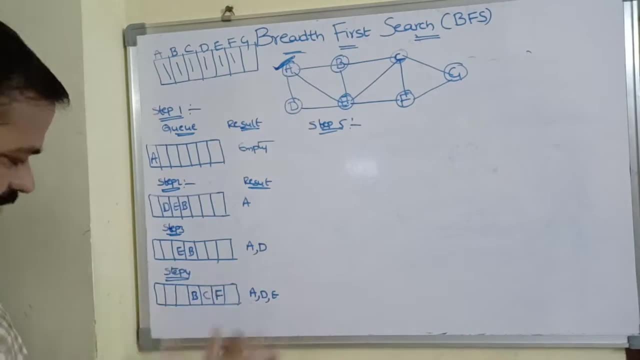 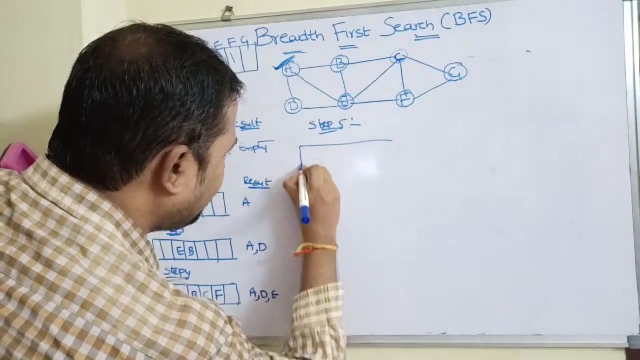 so make their status as visited. okay. and now let's write the next step. so step five, step five. so what is step five? same process, while the q is not empty. so here the q is not empty, so delete an element from the q so we have totally how many nodes? we have seven nodes with the q, so one, two. 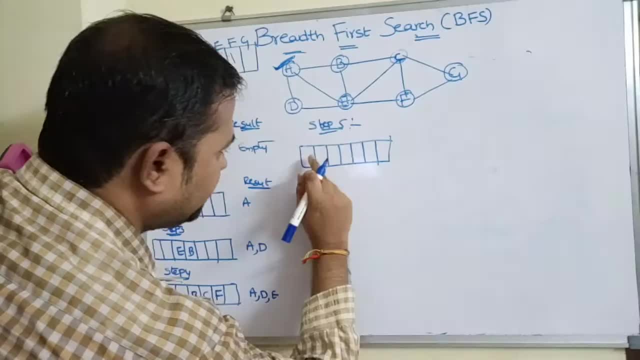 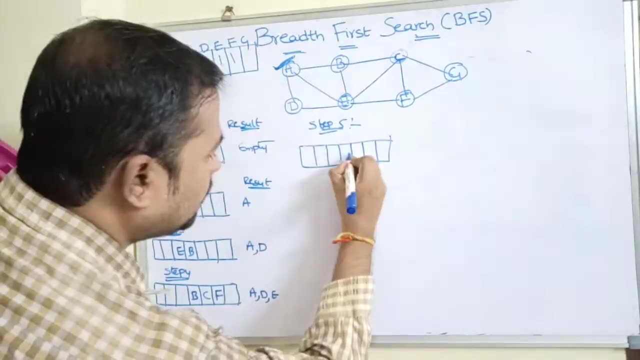 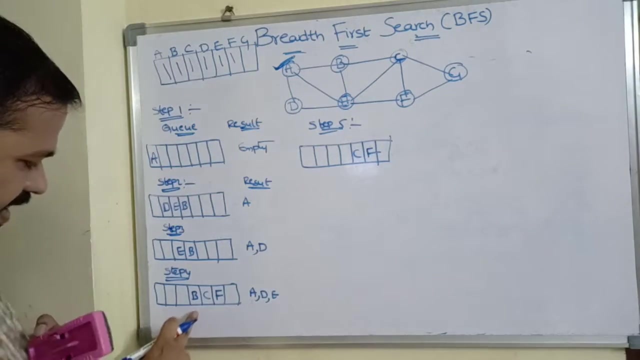 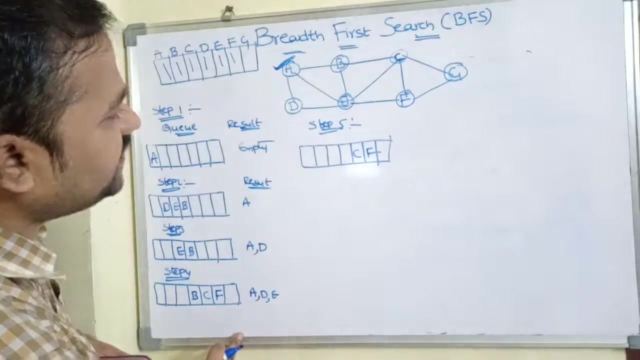 three, four, five, six. one, two, three, four, five, six, seven. so we have to delete b now. so delete b from the q and insert all the unvisited adjacent vertices of the b into the q. so what are the unvisited adjacent vertices of the b here? the adjacent vertices of the b are c and b. 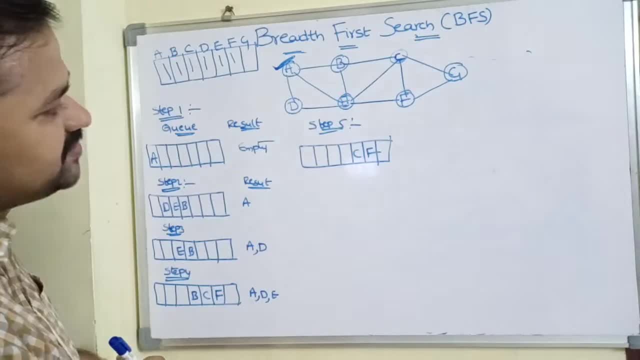 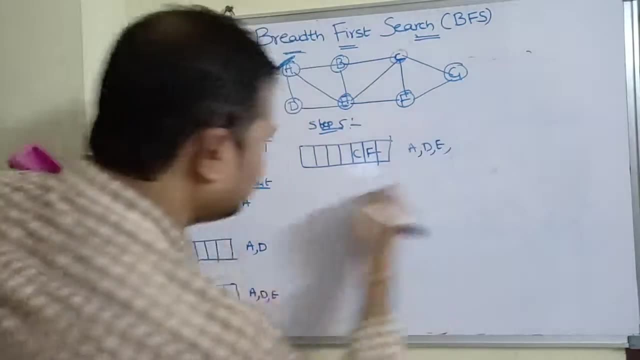 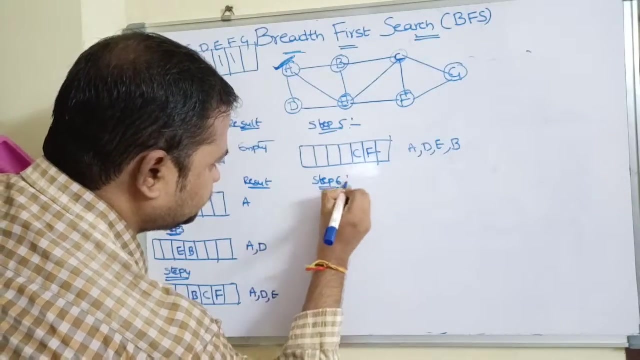 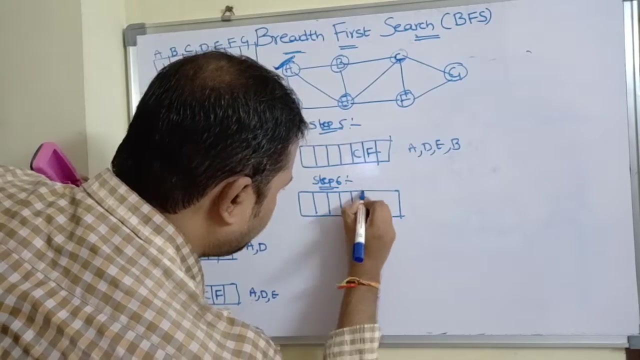 c is already visited as well as e is already visited, so there is no need to perform any nq operation now. so a, d, e, a, d e. so b is deleted from the q, so display that one. okay, so next step, step six. so delete an element from the q. so one, two, three, four, five, six, seven. so the c is deleted from the. 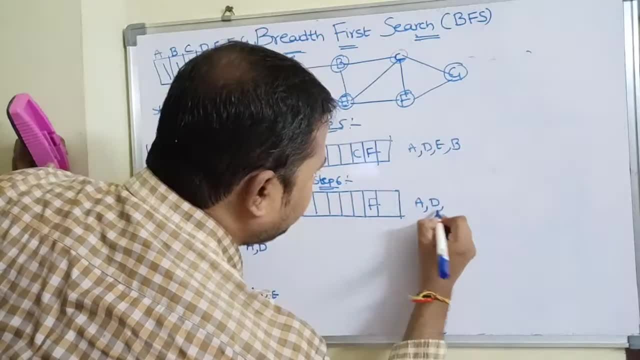 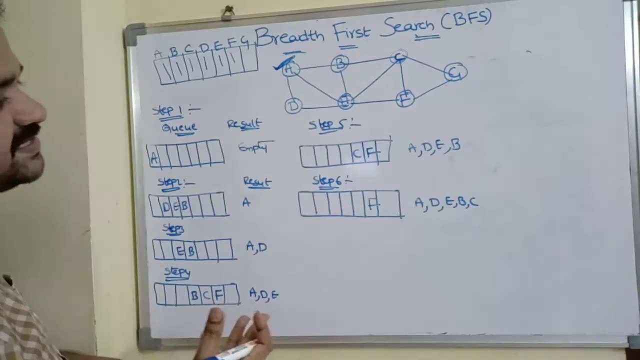 q. okay, and print it. it specifies that we have visited that node, so print it. so next we have to insert unvisited adjacent vertices of c into the q. so what are the adjacent vertices of c, f and g? so f is already visited, but g is not visited, so we have to insert unvisited adjacent vertices. 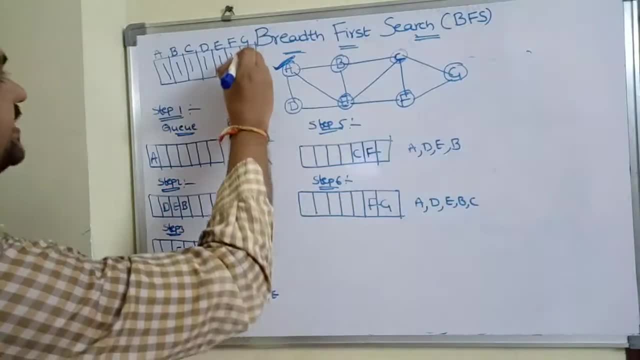 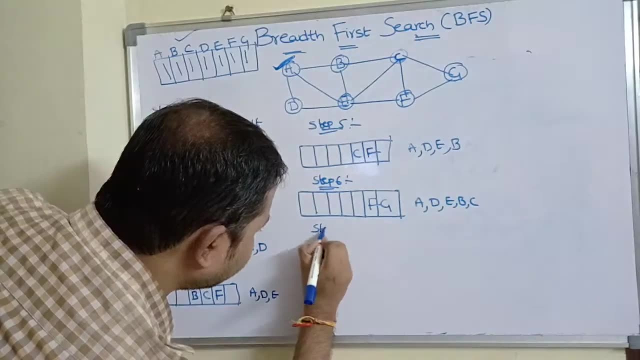 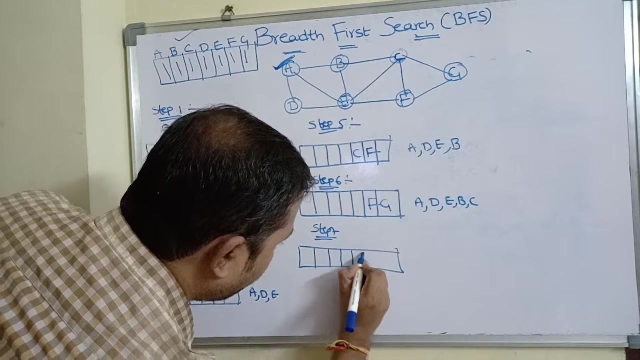 of c into the q. so insert g into the q and make g status as visited. so it specifies that now all the nodes and vertices are visited. okay, so let us perform the next step. step seven. so we have a q with seven nodes. so one, two, three, four, five, six, seven. okay, next we delete an element from the q. 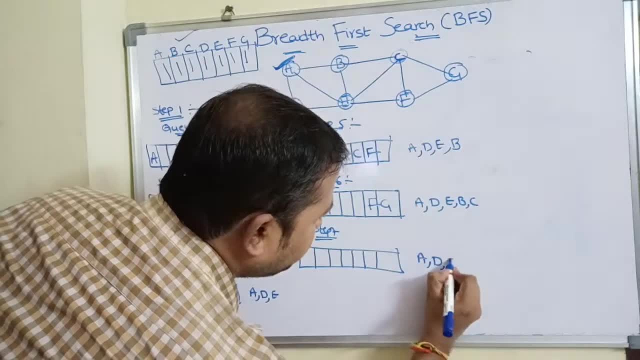 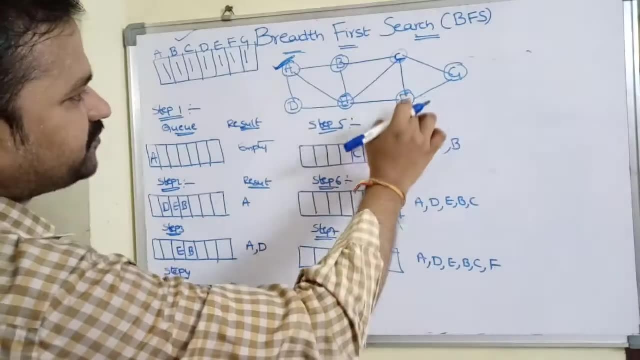 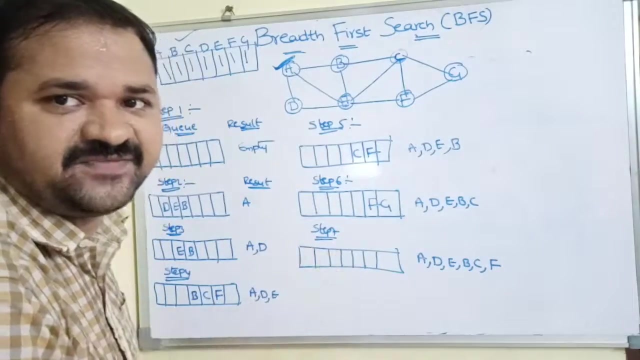 so the starting element is f, so f is deleted from the q. so a, d, e, b, c, so i'm gonna print it. so what are the adjacent vertices of f", c, e and g? but all the nodes are visited, so there is no unvisited the adjacent vertices. 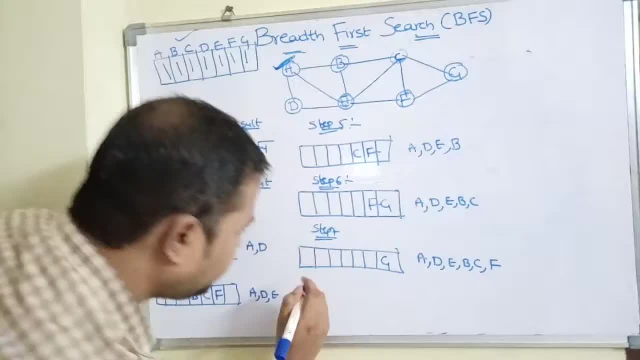 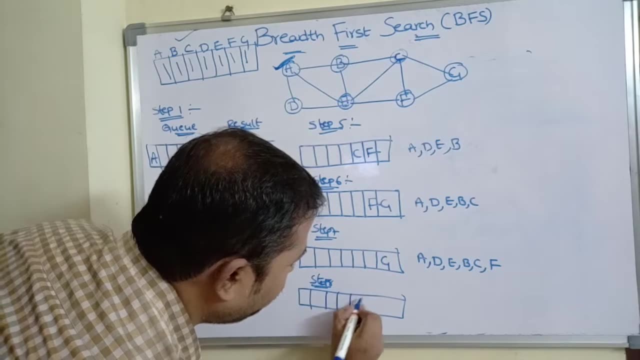 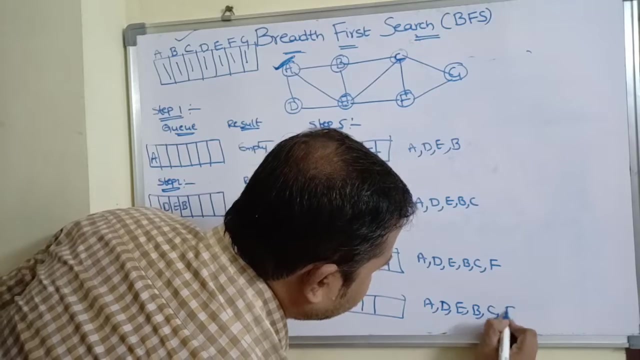 so there is no need to perform any enqueue operation. so likewise, perform the last step, step eight. so one, two, three, four, five, six, seven. okay, so delete g from the q. so a, d, e, b, c, f, g display it and there are values that are lost for priority: one, two, three, four, five, six, seven. okay, so delete g from the q. so a, d, e, b, c. if g, dah bye and there are no escaped notes.